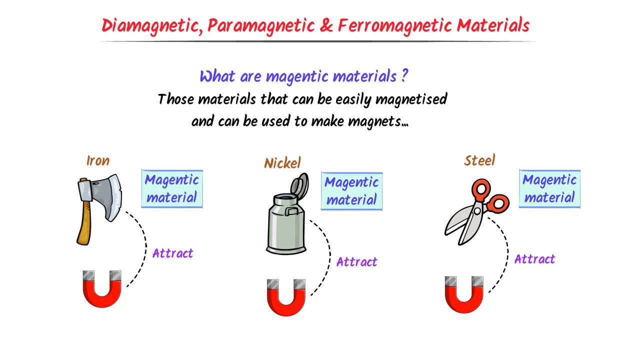 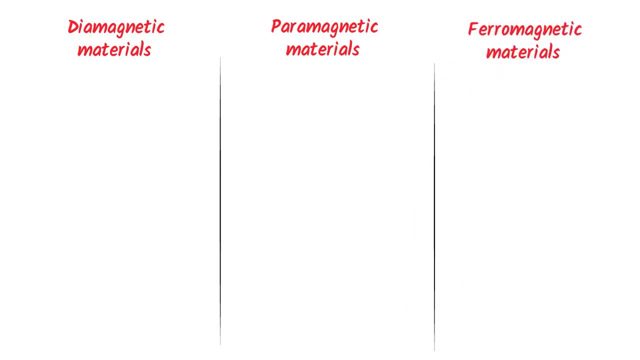 Now there are three primary categories of magnetic materials, like dimagnetic materials, paramagnetic materials and ferromagnetic materials. Dimagnetic materials are those materials which are weakly repelled by a magnet. For example, when you place gold in a magnetic 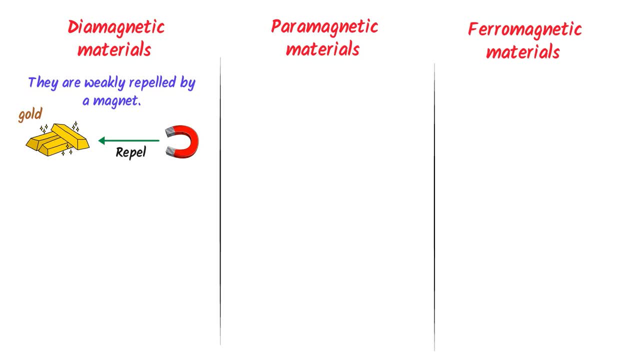 field, it is weakly repelled by the magnet, While paramagnetic materials are those materials which are weakly attracted by a magnet. For example, when you place aluminum in a magnetic field, it is weakly repelled by the magnet. For example, when you place gold in a magnetic 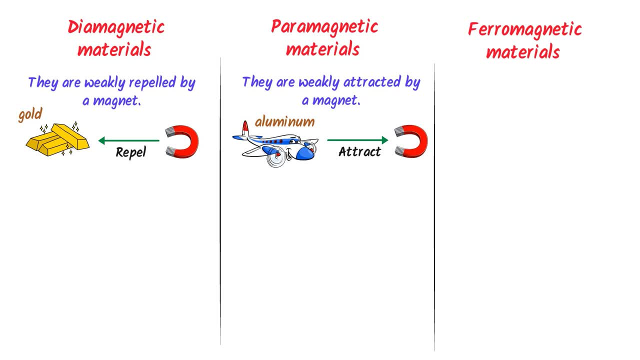 field, it is weakly attracted by the magnet, While ferromagnetic materials are those materials which are strongly attracted by a magnet. For example, when you place iron in a magnetic field, it is strongly attracted by the magnet. Secondly, if you place diamagnetic materials, 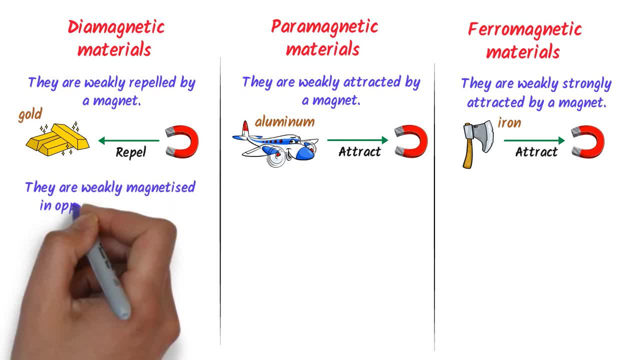 in a magnetic field, they are weakly magnetized in the opposite direction of the magnetic field. For example, if the magnetic field is magnetized, then iron is magnetized in field is in this direction, then diamagnetic materials are magnetized in opposite direction. 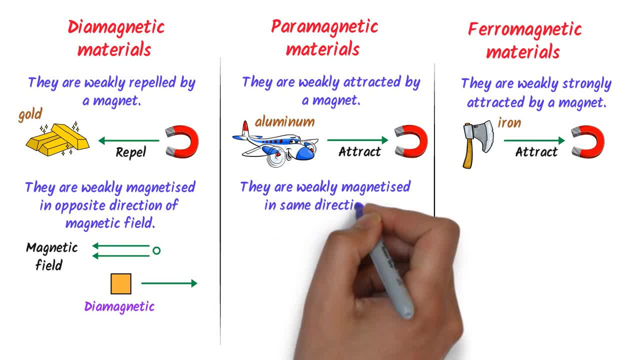 while paramagnetic materials are weakly magnetized in the same direction of magnetic field. For example, if the magnetic field is in this direction, then diamagnetic materials are magnetized in the same direction, while ferromagnetic materials are also strongly magnetized in the same direction of magnetic field. 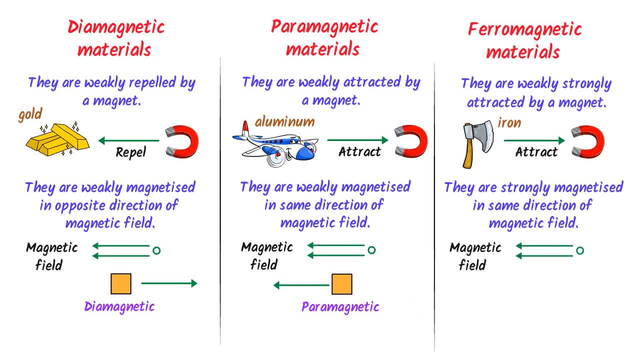 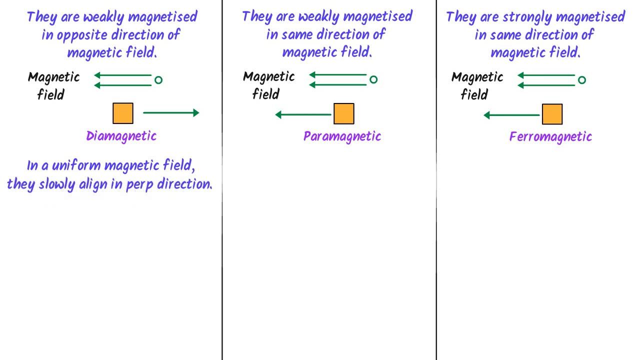 For example, if the magnetic field is in this direction, then ferromagnetic materials are magnetized in the same direction. Thirdly, when a diamagnetic rod is freely suspended in a uniform magnetic field, it slowly aligns itself in a direction perpendicular to the applied magnetic field. 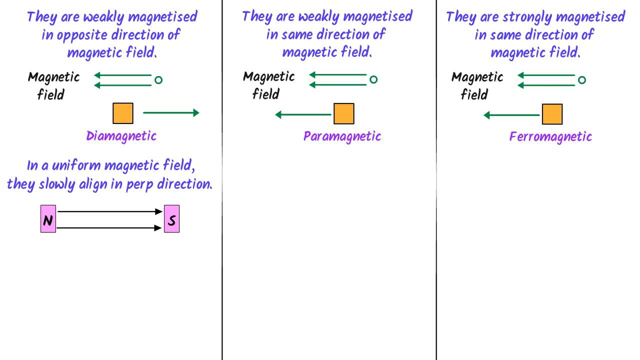 For example, magnetic field is in this direction. The diamagnetic rod will slowly align itself in a perpendicular direction. When a paramagnetic rod is freely suspended in a uniform magnetic field, it slowly aligns itself parallel to the applied magnetic field. For example, magnetic field is in this direction. 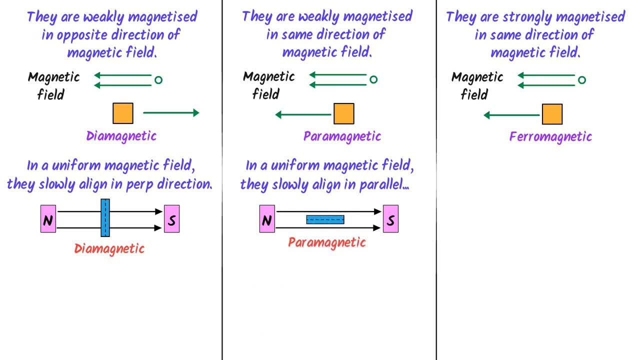 The paramagnetic rod will slowly align itself parallel to the applied magnetic field. and a uniform magnetic field? it quickly aligns itself parallel to the applied magnetic field. For example, magnetic field is in this direction. the ferromagnetic rod will quickly align itself. 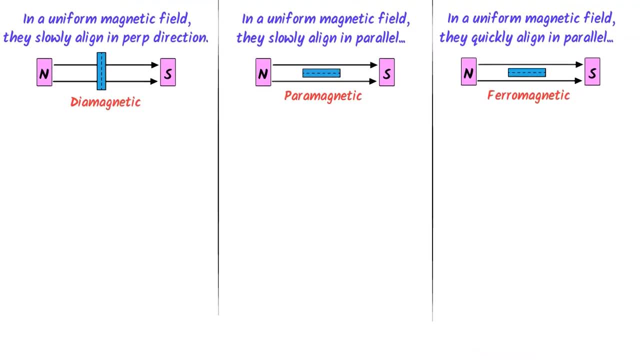 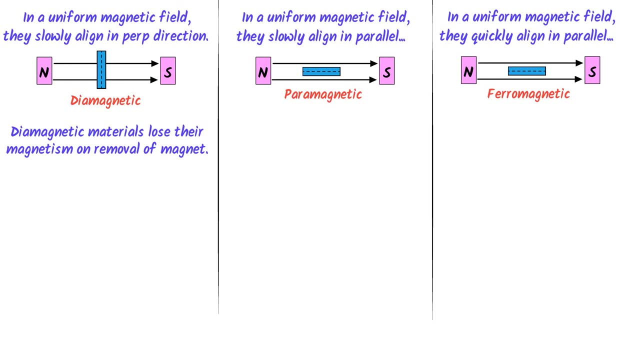 parallel to the applied magnetic field. Fourthly, dimagnetic materials lose their magnetism on removal of external magnetic field, while paramagnetic materials also lose their magnetism on removal of external magnetic field, while ferromagnetic materials do not lose their magnetism on removal of external 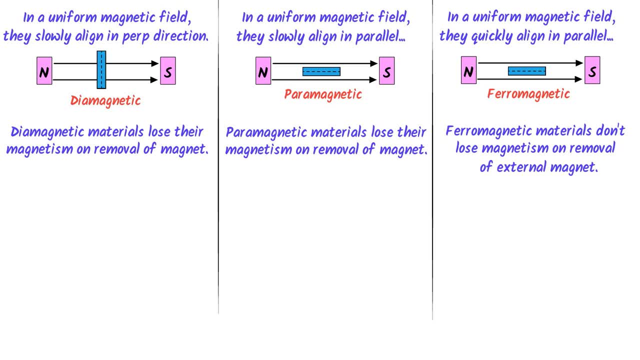 magnetic field. Remember that they are permanent magnet. Fifthly, in a non-uniform magnetic field, the dimagnetic materials move from a stronger to a weaker field due to repulsion. For example, in the non-uniform magnetic field, these dimagnetic materials move from: 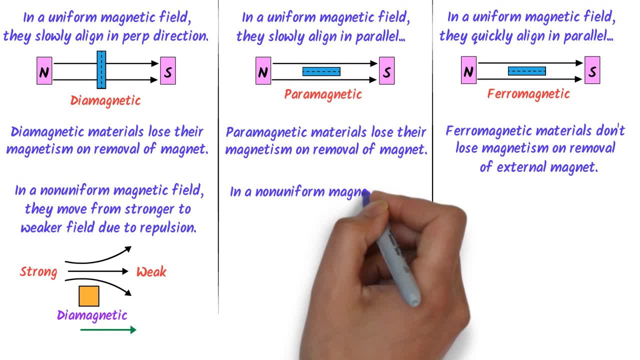 a stronger to a weaker field, While in a non-uniform magnetic field, the paramagnetic materials move from a weaker to a stronger field with a weaker traction. For example, in this non-uniform magnetic field, the paramagnetic materials move from a weaker to a stronger field due to weak attraction. 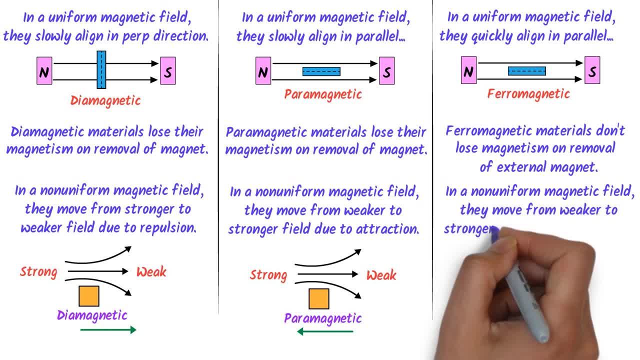 While in a non-uniform magnetic field, the paramagnetic materials move from a weaker to a stronger field due to weak attraction. For example, in the non-uniform magnetic field, the dimagnetic materials move from a weaker to a stronger field due to strong attraction. 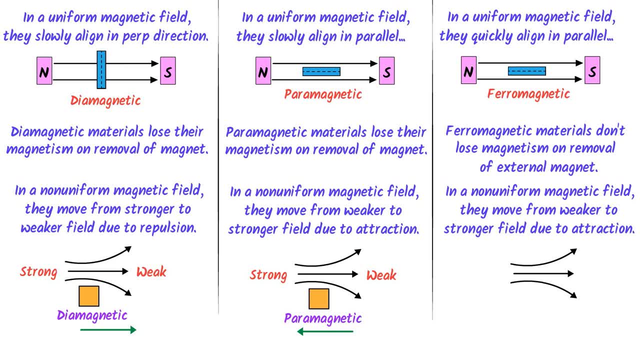 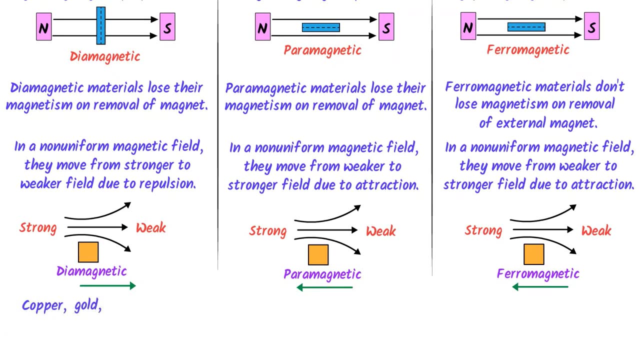 For example, in the non-uniform magnetic field, the paramagnetic materials move from a weaker to a stronger field due to strong attraction. Sixthly, the examples of dimagnetic materials are copper, gold, silver, water, air, argon.